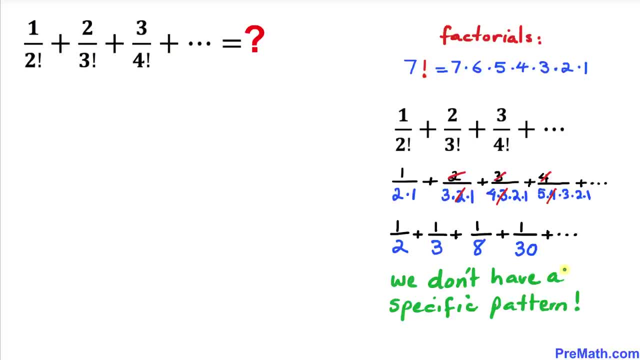 series does not give us any clear pattern. therefore, we are going to think outside the box and take a different approach. so let's go ahead and manipulate this infinite series. let's focus on these and numerators: 1. I can write 1 as 2 minus 1. likewise, 2 could be written as 3 minus 1, and this 3 could be. 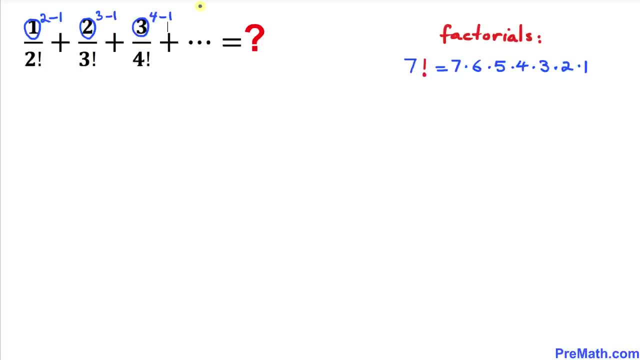 written as 4 minus 1. on and on and now, in this next step, I have replaced this 1 as 2 minus 1. this 2 I replaced by 3 minus 1, likewise 3 by 4 minus 1. now, in this next step, let's go ahead and split this. 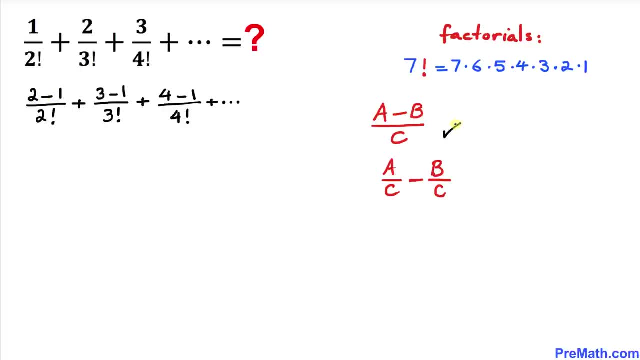 frame by 2. and now, in this next step, let's go ahead and split this frame by 2 fraction into two fractions by using this rule, so this could be written as 2 divided by 2 factorial minus 1 divided by 2 factorial plus, likewise, 3 divided. 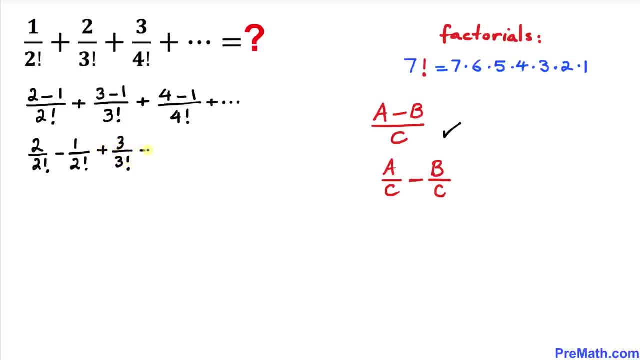 by 3 factorial minus 1 over 3 factorial plus. 4 divided by 4 factorial minus 1 over 4 factorial and plus goes on and on and on, and now let's focus on these fractions: 3 divided by 3 factorial and this one, 4 divided by 4. 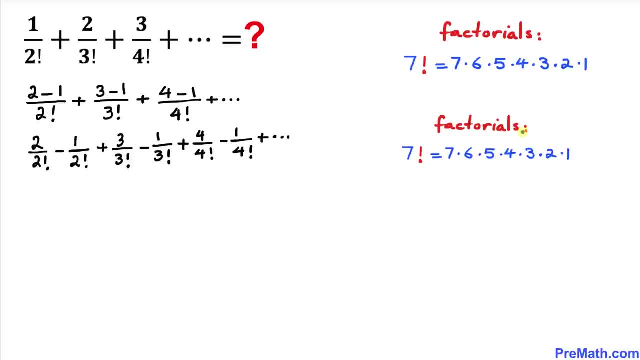 factorial. before we go any further, let's talk about this example once again: 7 factorial could be written as: 7 times 6 times 5 times 4 times 3 times 2 times 3 times 1- let's focus on this part- 6 times 5 times 4 times 3 times 2 times 1, so this: 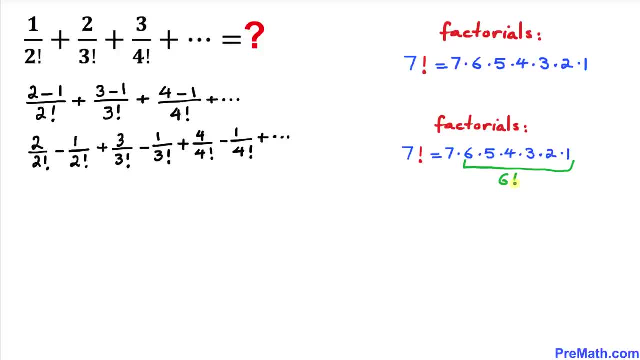 is same as could be written as 6 factorial. so therefore we can write this 7 factorial as 7 times 6 factorial. so therefore we can write this 3 divided by three factorial as three divided by three times two factorial. and now you can see three and three. they cancel each other out, so this is same as writing one.